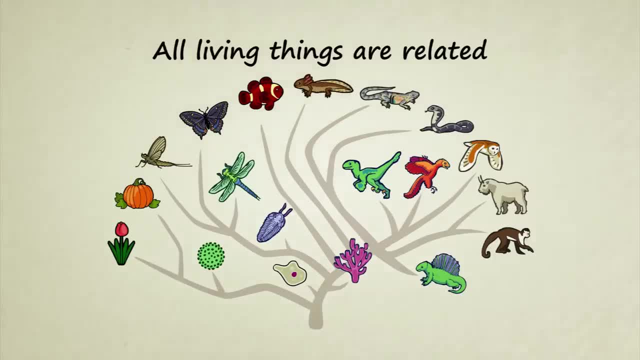 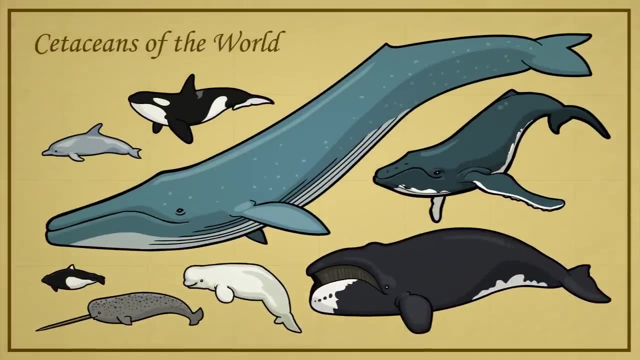 claim that all living things on earth are related. we can't not tackle the entire tree of life at once- after all, there's an estimated 8.7 million species alive today- so instead, we'll focus most of our attention on one fairly small but fascinating branch of the evolutionary tree: cetaceans. this branch includes whales. 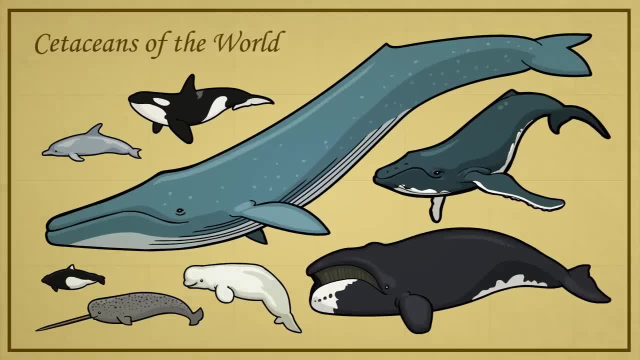 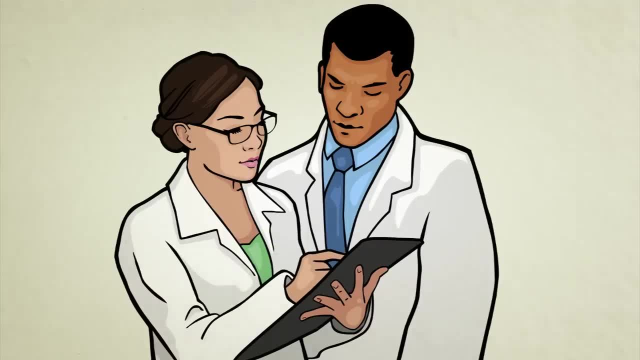 dolphins and porpoises. biologists tell us that all these creatures are closely related and that the entire group evolved from an ancient four-legged land mammal. instead of taking their word for it, they are related to each other. they are related to each other. they are related to each. 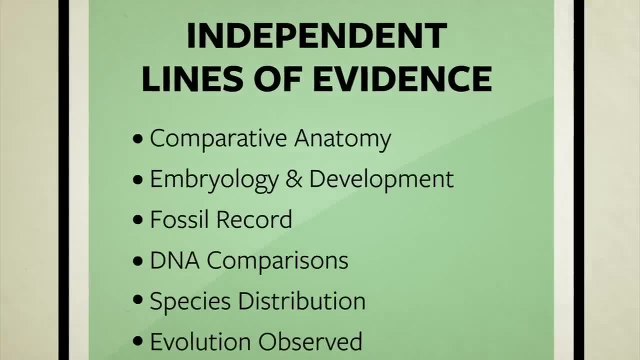 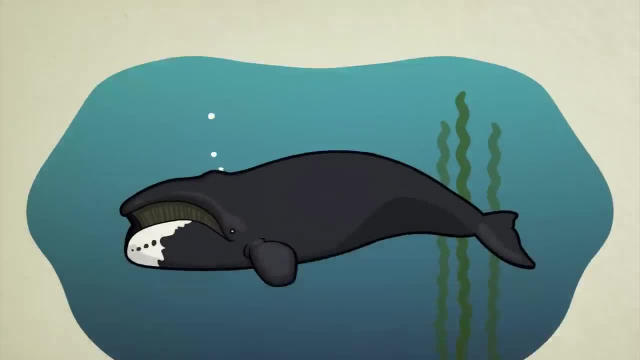 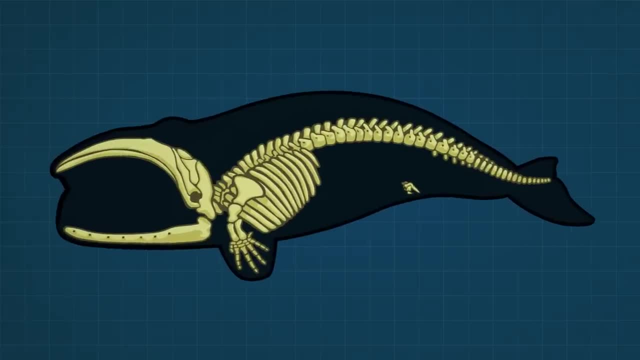 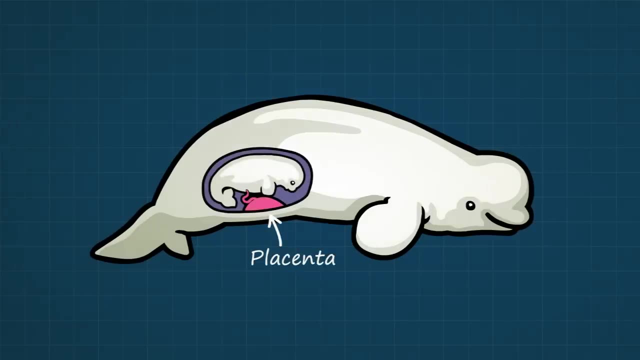 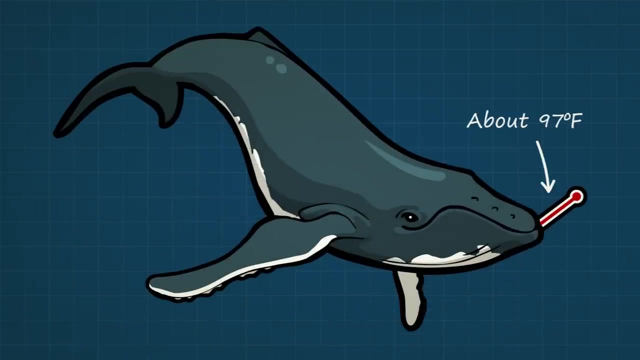 a close inspection of their anatomy, however, tells us a very different story. whales, just like land mammals, but, unlike fish, have placentas and give live birth. they feed milk to their young. they are warm-blooded, which is extremely rare for a fish, and whales do not have gills, instead just 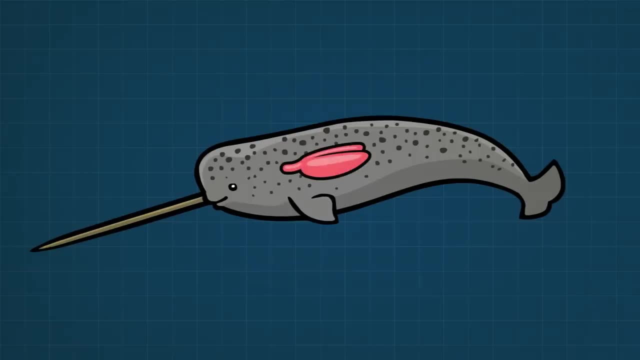 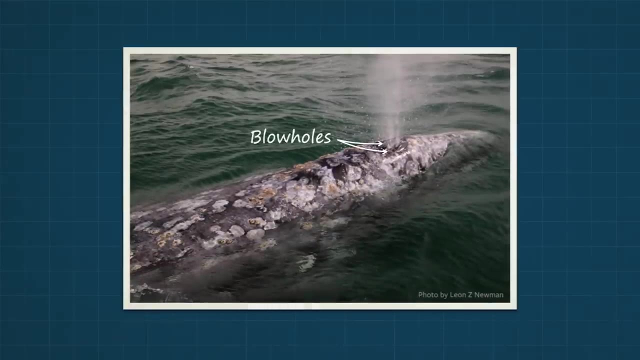 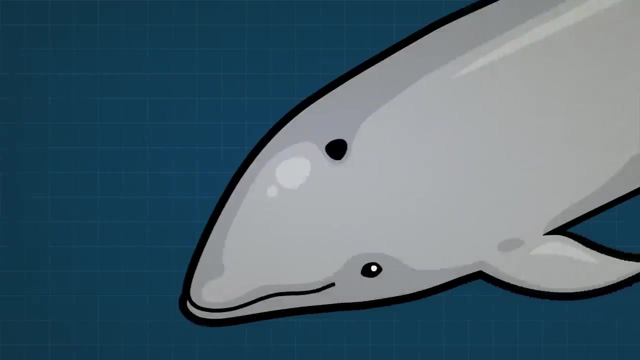 like us, they breathe air with two fully developed lungs. whales don't seem to have noses like mammals do. instead, they breathe through blowholes coming out the tops of their heads. some whales have two blowholes, which almost look like nostrils, but dolphins and porpoises only have one, surprisingly, 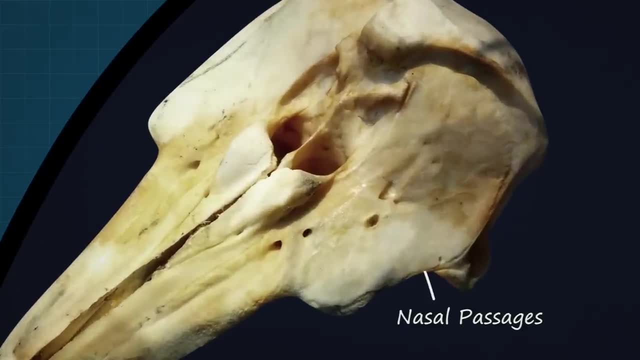 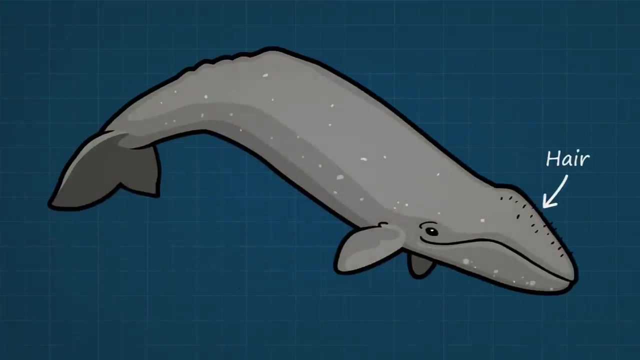 if you look at their skulls, you find that the blowhole splits into two nasal passages inside the head. could it be that the blowhole is actually a highly modified mammal nose? it looks that way, but we'll need more evidence to be sure. many whales have hair, just like land mammals in this. 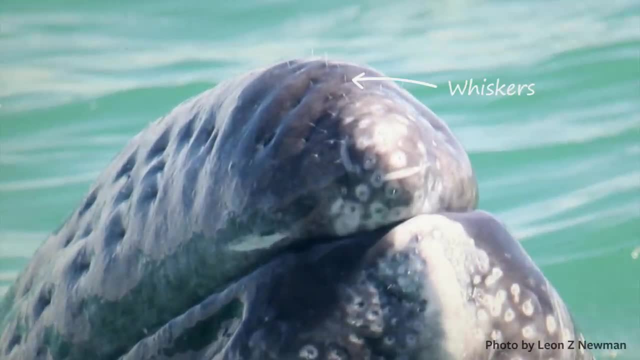 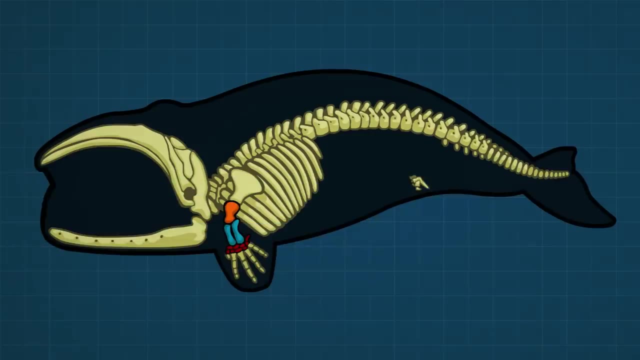 photograph you can actually see the whiskers of this baby gray whale as he rests his chin on Mama's back. strangely, whales have more poppy hair, just like land mammals, than mostdoo whales seem to. zwei Whales have arm, wrist, hand and finger bones inside their front flippers. 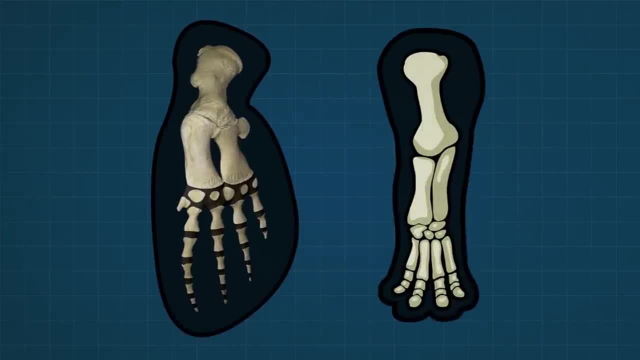 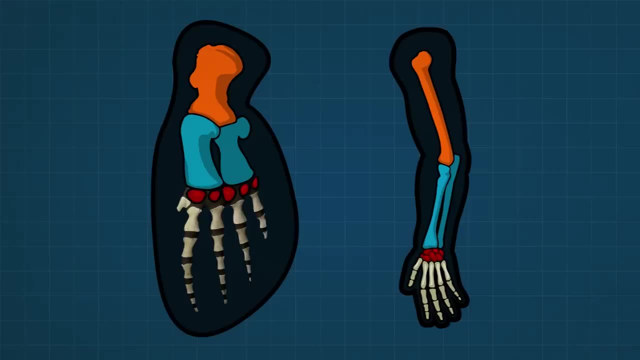 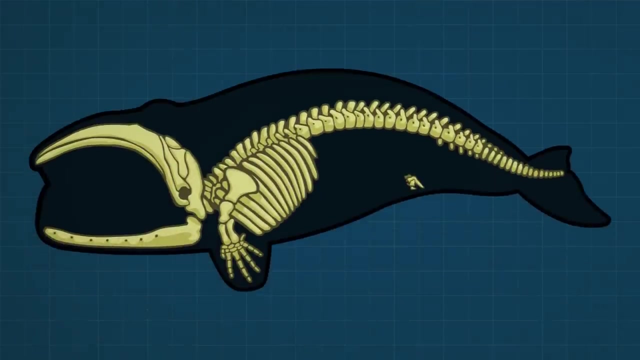 Here's a photo of these bones, the same bones that bats, hippos and people have in their front appendages. One bone, two bones: wrist, hand and finger bones. Modern whales do not have back legs, but they do have a strange pair of bones where the 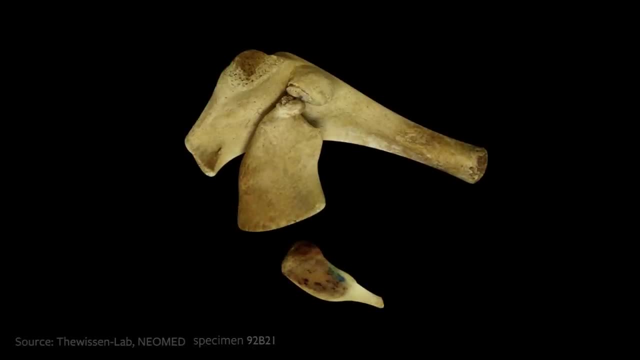 hind leg should be. Here's a picture of these bones from a bowhead whale. They almost look like shriveled hip, thigh and shin bones. This one even has a ball and socket joint between the hip and thigh bone, just like. 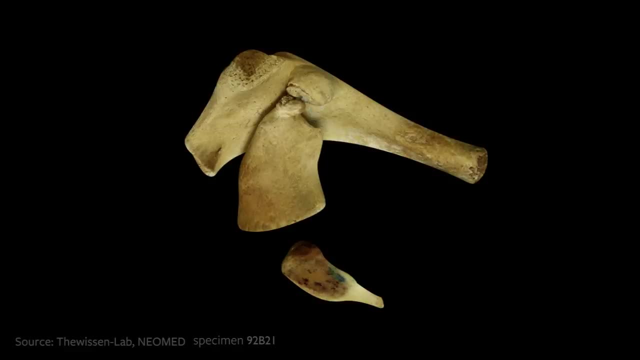 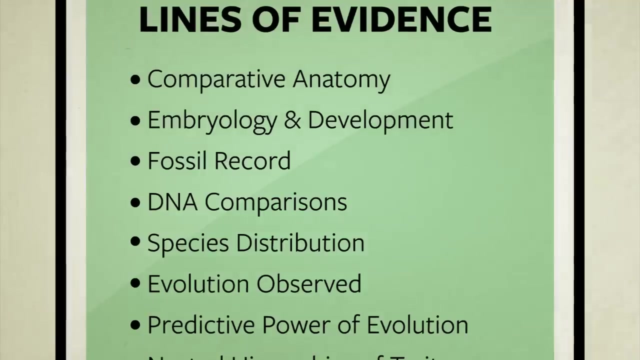 the ball and socket joint in your own hip. Is this resemblance a mere coincidence, or are these real leg bones, perhaps leftovers from the whale's evolutionary history? Before we draw any bold conclusions, let's see if a completely separate line of evidence will confirm our suspicions. 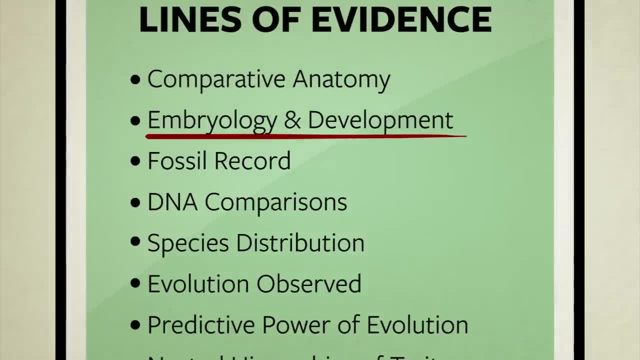 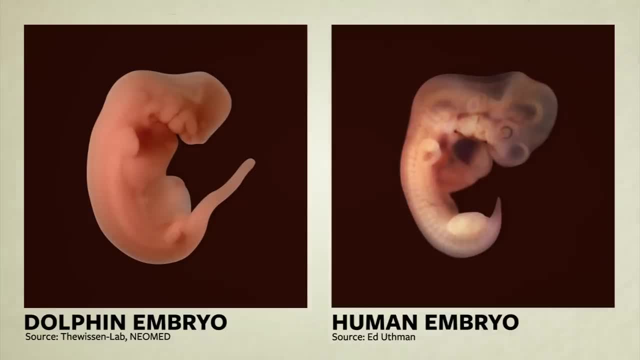 1. Embryology is the study of how creatures develop before being born or hatching from an egg. Here we see a dolphin and a human embryo side-by-side at similar stages of development. Notice that they both have what look like arm buds and leg buds. 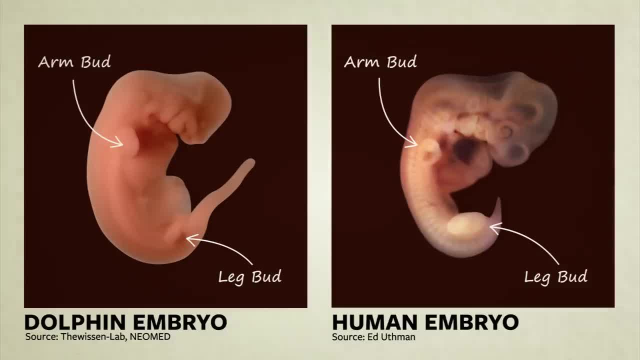 In humans, the leg buds grow to become legs. In whales, they grow for a while but then stop effectively fading away as the rest of the whale continues to grow. 2. In humans, the leg buds grow to become legs 3. 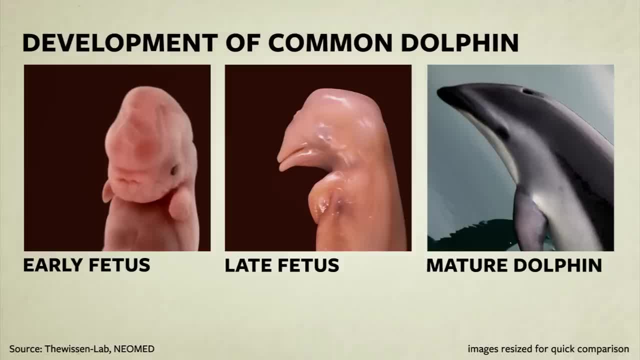 In persons. they grow for a while but then stop quite a bit later to open, essentially modeled like little agrees of a dropped nose. To say that there are no pup from another planet is a huge上 in the history of human life. 1.. 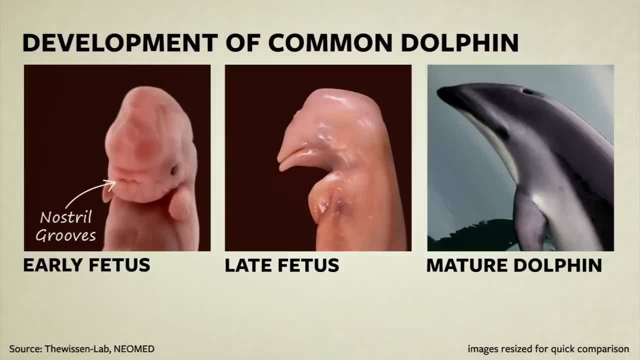 In humans, animals grow from their mulheres. 2. In humans, animals grow from their mares. 3. In humans, animals grow from their laissez-faire environments. 4. bowls grow from their ladies, like the ones on willow orное. 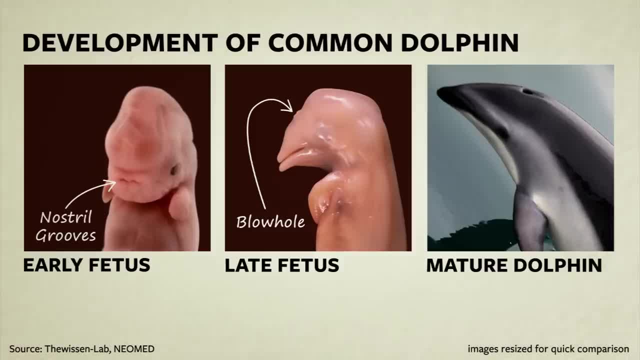 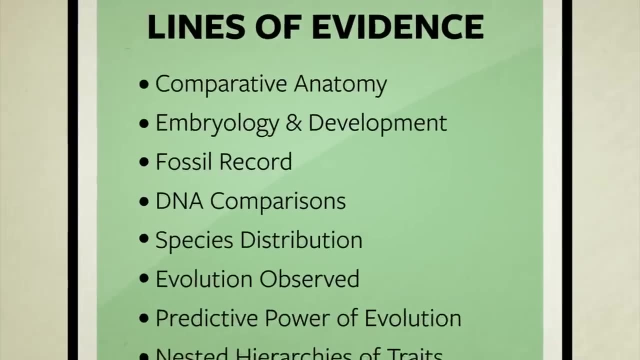 6. Living life can be complex. Thus, this is what happens when you pick theranium: Familia milk your voz полож 其實baren H recalls a verbe: The ancestors of whales were once four-legged land creatures. Will the fossil record act as a third witness confirming this idea? 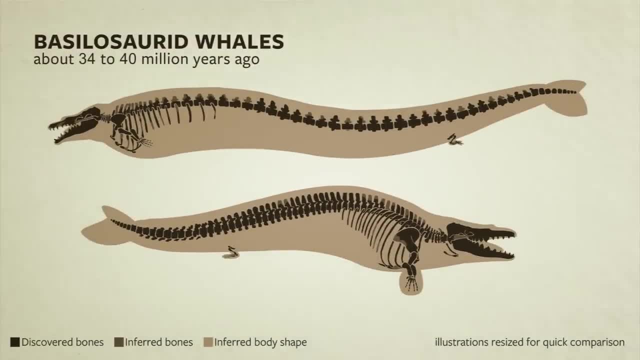 These are two species of extinct basilosaurid whales. These animals are known for multiple, well-preserved skeletons and they appear to have lived side by side roughly 34 to 40 million years ago. In this photograph, we're looking down at the top of a basilosaurid skull. 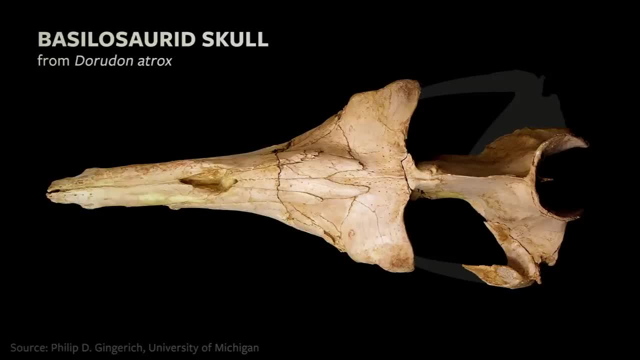 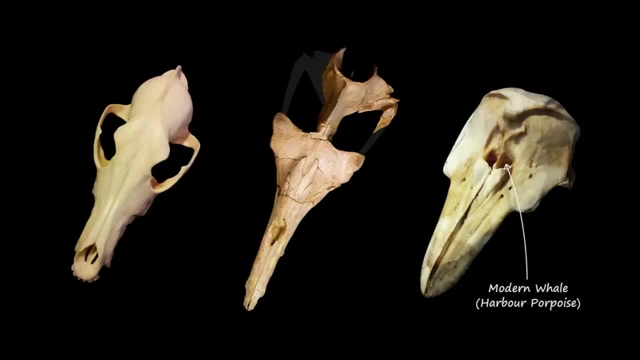 This is not a model or a cast. These are the actual bones which were pulled from the ground. Notice that the nasal opening is not on the top of the head, like those of modern whales, and not at the end of the snout, like those of land mammals. 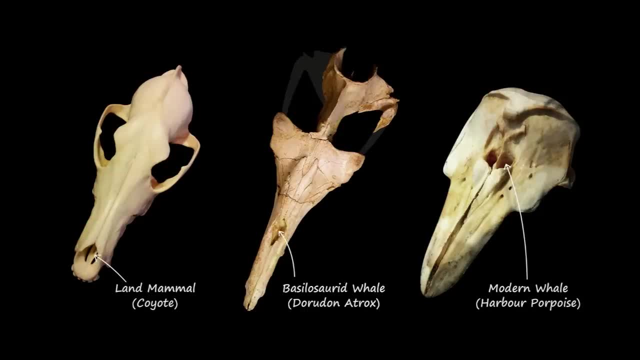 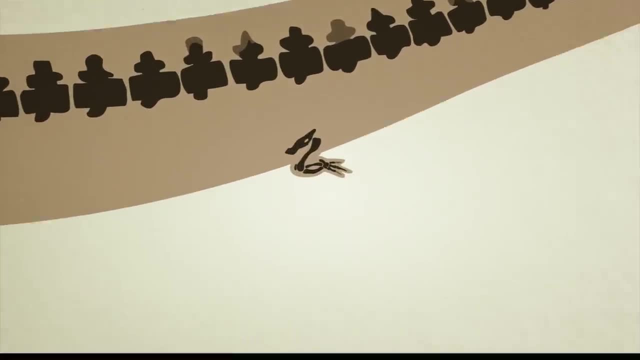 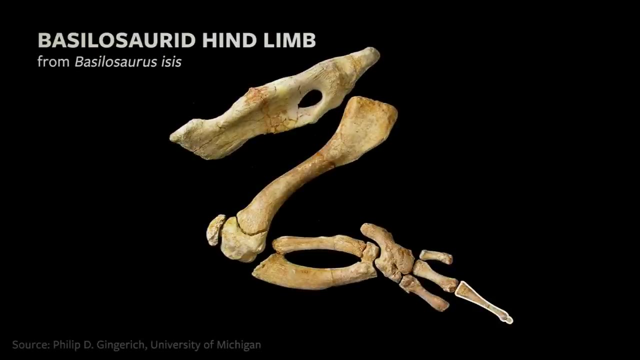 Instead, it's right in the middle. This is an intermediate species, exactly what evolution tells us we should find. At the back end of a basilosaurid's body there are small yet fully developed hips, legs, ankle feet and toe bones. 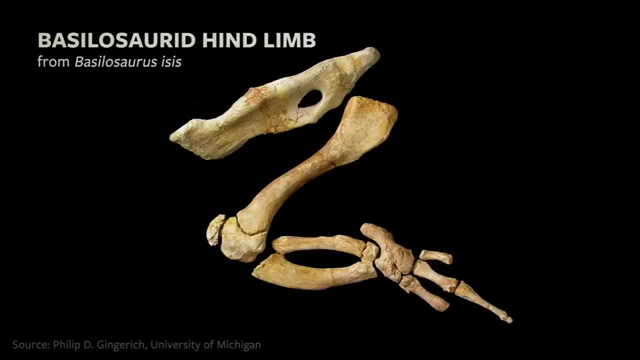 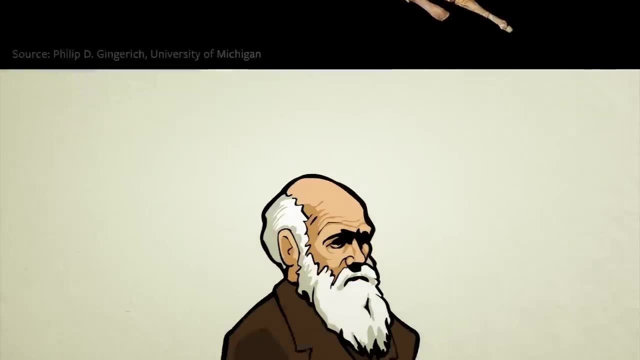 These legs are far too small for walking on land, but they may have been useful while mating or for scratching away parasites and itchy skin. Evolutionary theory tells us that the further we go back in time, the harder it should be to distinguish whales from normal land mammals. 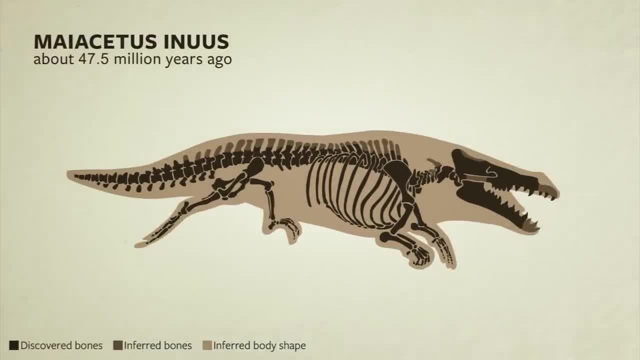 Meet Myocetus. The hip bones of Myocetus seem sturdy enough to walk on land, but this animal is considered to be a whale for many reasons. Their skeletal structure is very similar to that of a human. The skeletons have all been found among fossils of sea creatures. 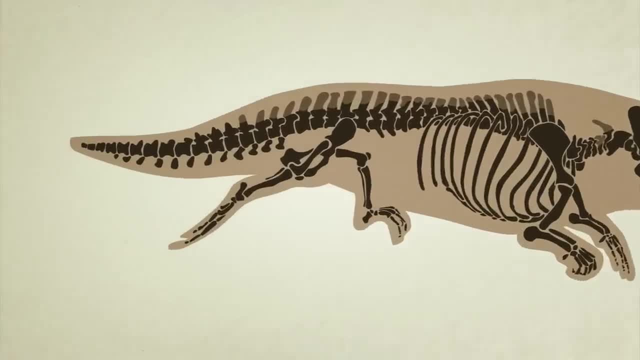 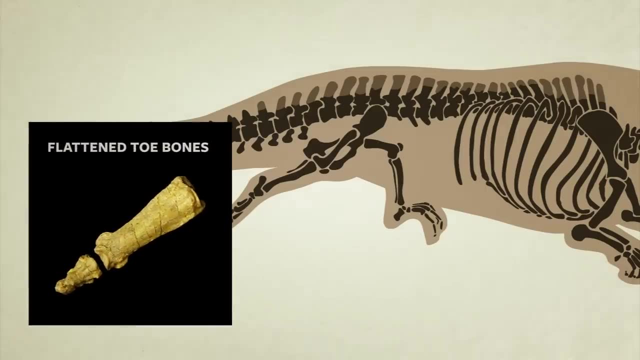 which tells us they lived in the ocean. Their short legs, combined with long, flat fingers and toes, suggest they were strong swimmers with webbed hands and feet. Here we see the bottom side of a Myocetus' jaw and skull. 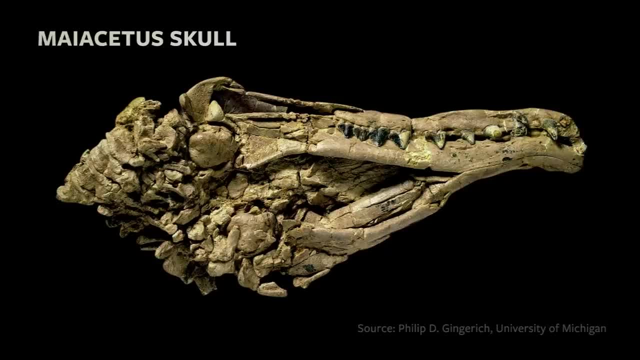 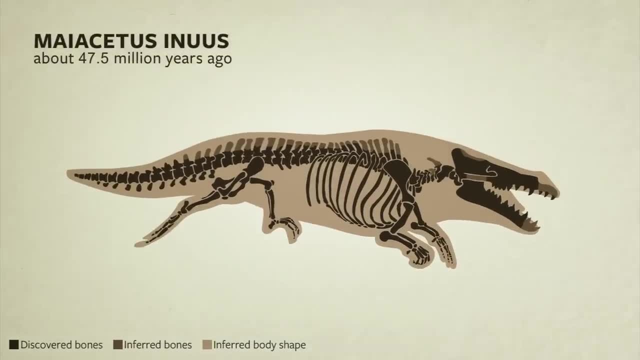 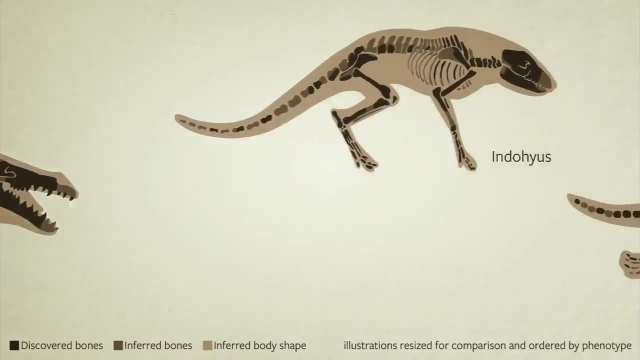 Her teeth match those of the basilosaurid whales we saw earlier, and the unique structures of her middle ear bones match those of basilosaurid whales and modern whales. Myocetus appears to be a walking whale. Scientists have found the fossils of many ancient whale-like mammals and continue to find more. 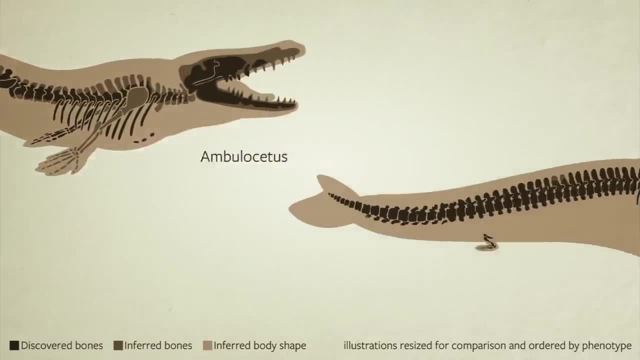 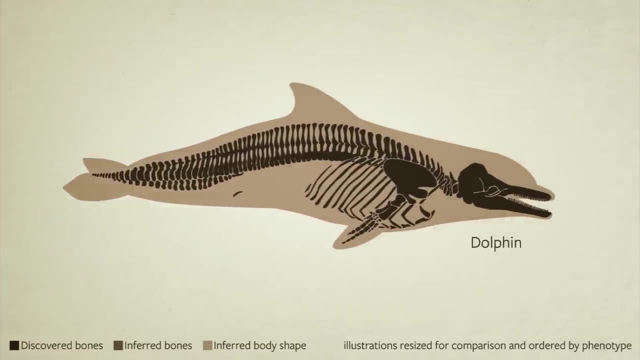 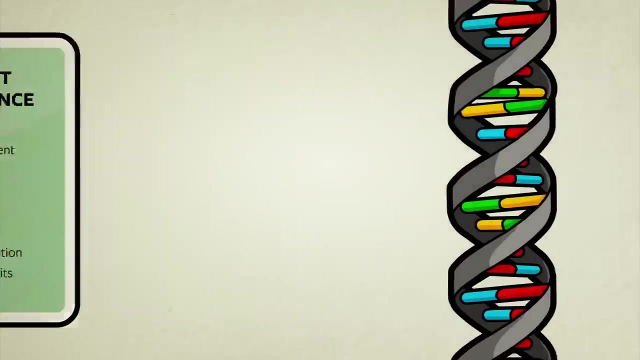 Together, these fossils blur the line between four-legged land mammals and fully aquatic modern whales, solidifying the idea that whales indeed evolved from land creatures. Now let's look at a fourth line of evidence: DNA. DNA molecules contain chemical codes which act like recipes for living things. 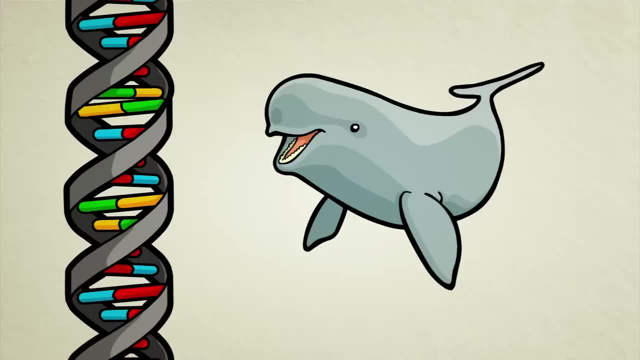 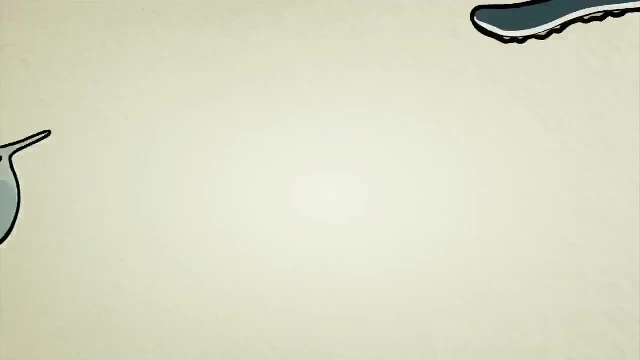 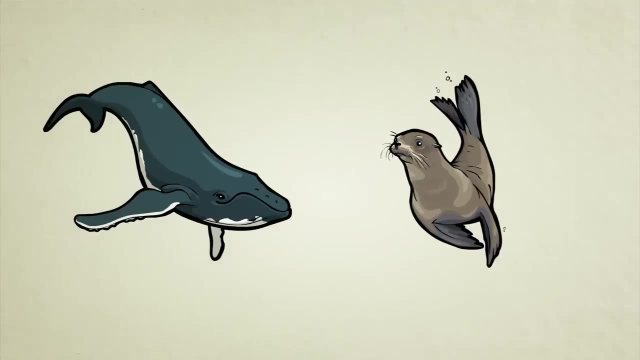 Without ever looking at bones, embryos or anatomy, researchers can compare the DNA code of different living creatures to find out who is most closely related to who. Whale DNA has been compared to all kinds of other animals- fish, sea lions, you name it- and so far the closest genetic match is to the pudgy. 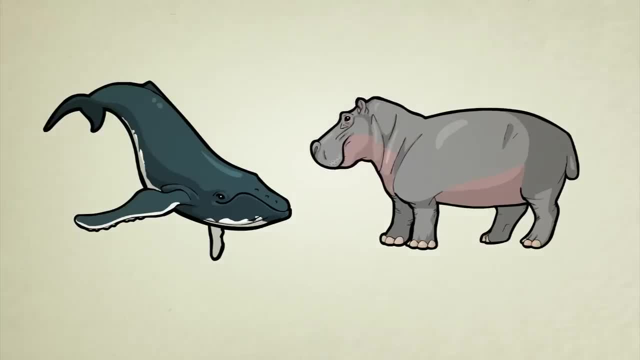 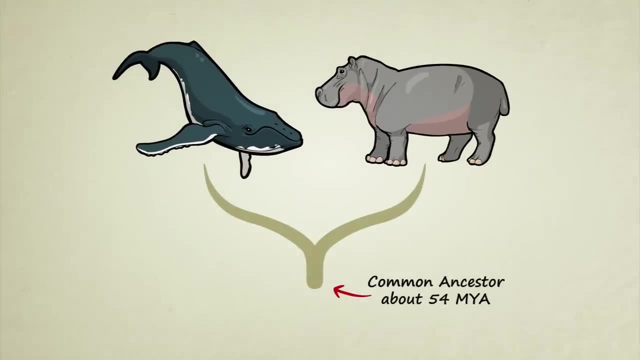 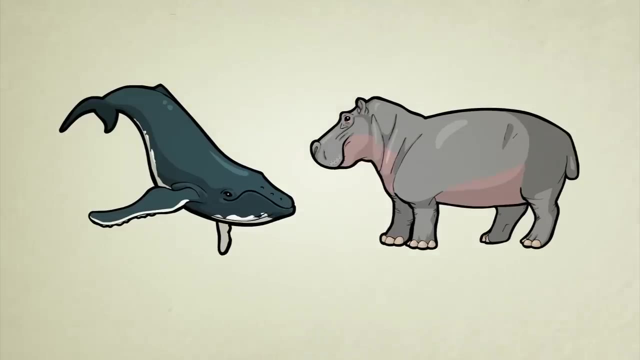 water-loving hippopotamus. This does not mean that whales evolved from hippos, But if this genetic finding is correct, whales and hippos both evolved from a common ancestor that lived roughly 54 million years ago At first. the link between whales and hippos surprised researchers. 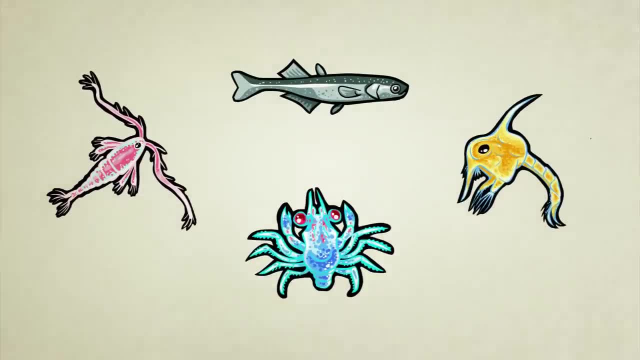 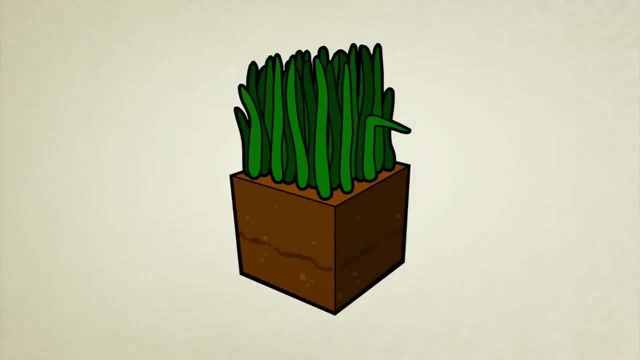 because whales are mainly carnivores: They eat things like fish and small crustaceans. Hippos, on the other hand, are mostly vegetarian. A closer look, however, reveals that hippos and whales actually share many strange features, some of which may have come from their 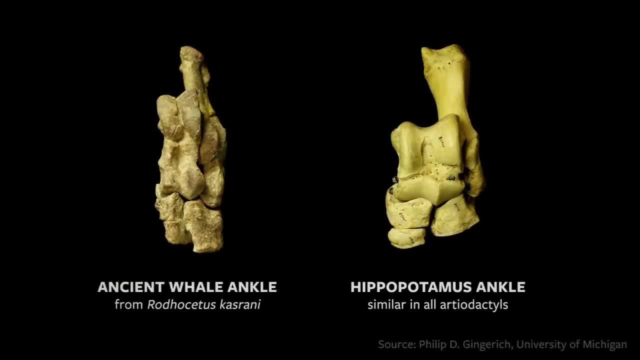 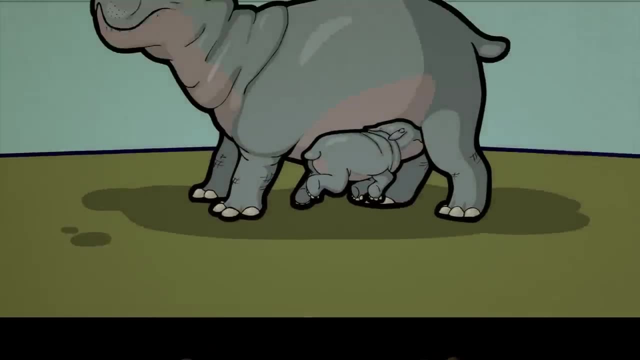 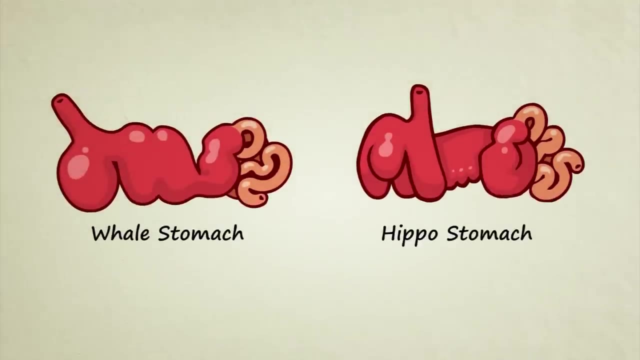 common ancestor, Ancient walking whales, have specially shaped ankle bones found only in hippos and the close relatives of hippos. Just like whales, hippos are known to give birth and even nurse their young underwater. They both have multi-chambered stomachs, which is common for herbivores but is almost unheard of. 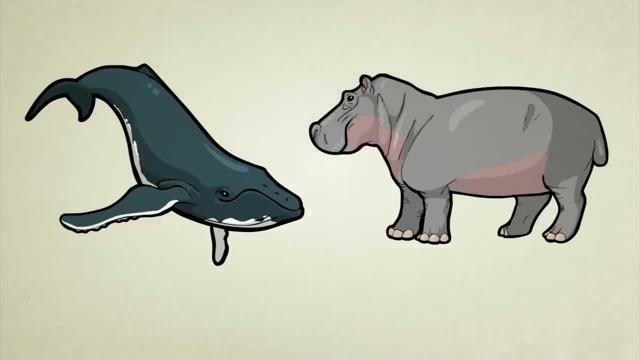 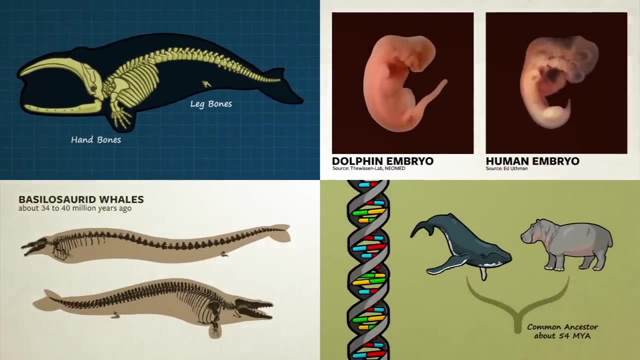 for meat-eating mammals. They are both missing a coat of fur. And here's a fun fact: whales and hippos are among the only mammals on earth that have internal testicles. So there you have it: four independent lines of evidence, all tell. 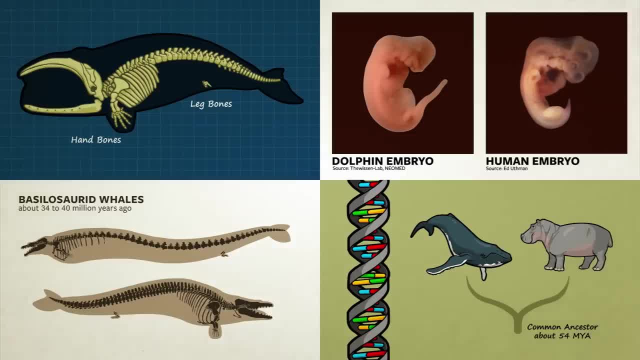 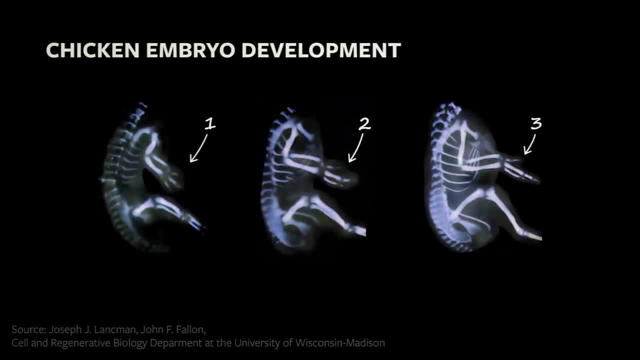 us the exact same story: Whales evolved from four-legged land mammals, But the history of whales is not the only evolutionary history that we've been able to work out. We know that the history of whales is not the only evolutionary history that we've been able to work out. 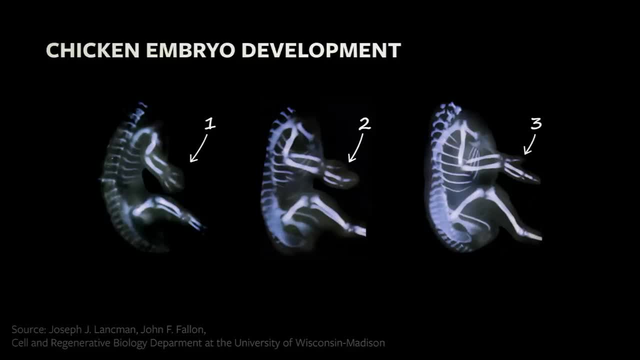 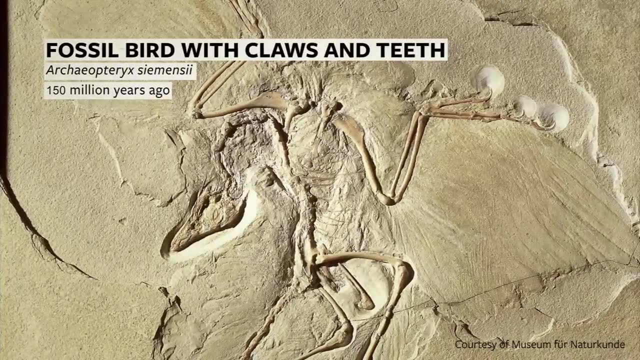 We know that the history of whales is not the only evolutionary history that we've been able to work out. We know from fossils, DNA, embryology and many other lines of evidence that bird wings are actually modified arms and claws. Birds evolved from dinosaur-like.